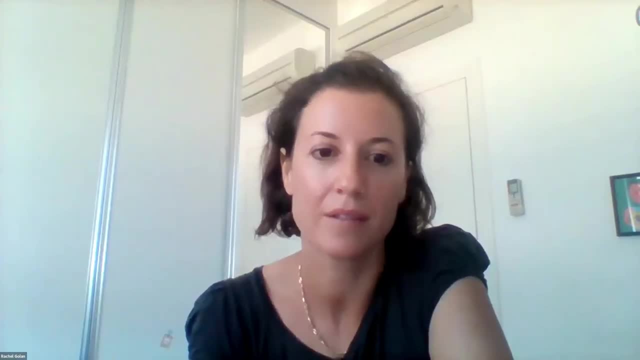 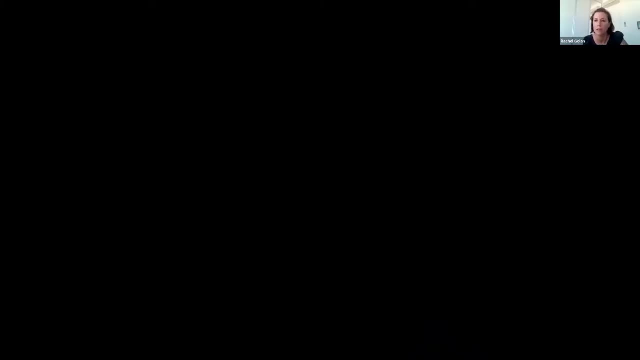 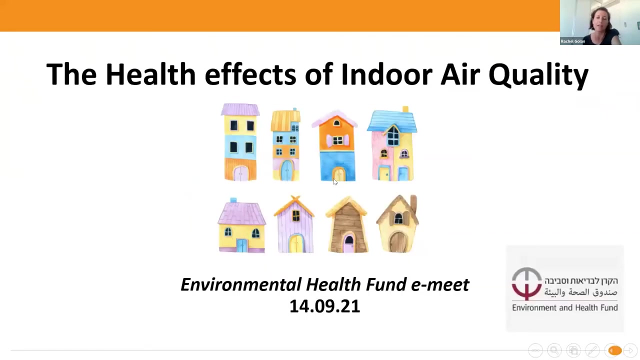 Thank you, Sorry for the introduction. There we go, All right, Okay, Good afternoon to everyone, And I'd just like to say thank you to the EHF for having this meeting and for getting us all together in this afternoon. So I must say, without knowing what the other 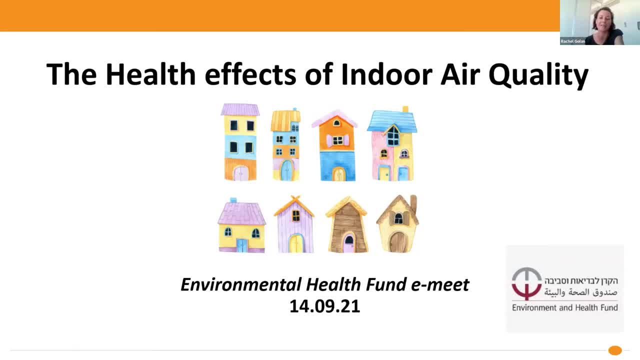 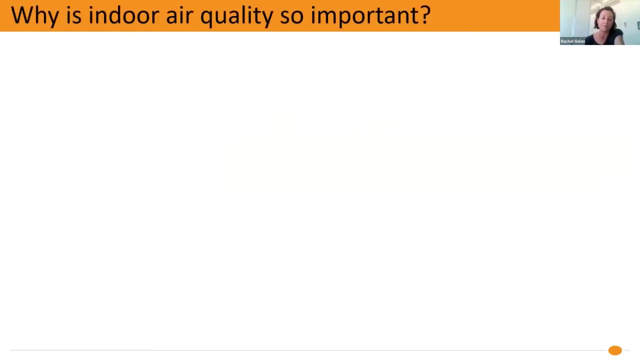 speakers will be talking about in detail, and I really love the thread that's going through our talks here and I'd like to zoom out a bit and talk about the health effects of indoor air quality And, as has been said an hour and a half ago, why is indoor air? 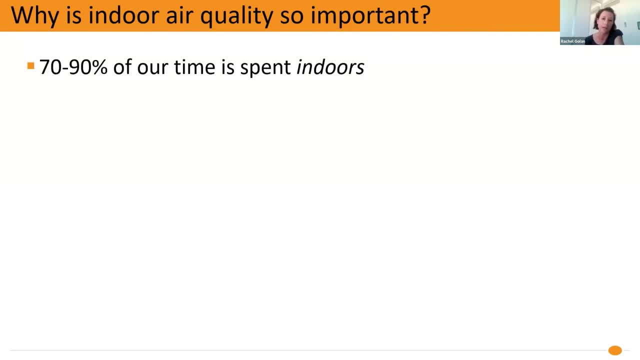 quality so important? It's because we spend most of our time in the air And we spend most of our time in the air, And we spend most of our time in the air And we spend most of our time indoors. And that's the answer for the question: We are spending our 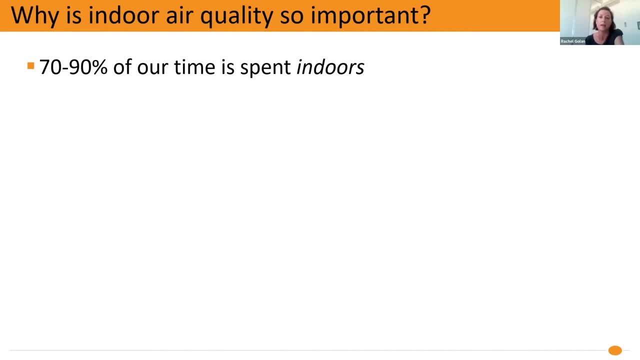 times, most of the days, especially in developed countries, but not only indoors, And therefore, although many studies, or maybe most of the studies and most of the knowledge that we have today is about ambient air pollution, at the end of the day, most of our time we're 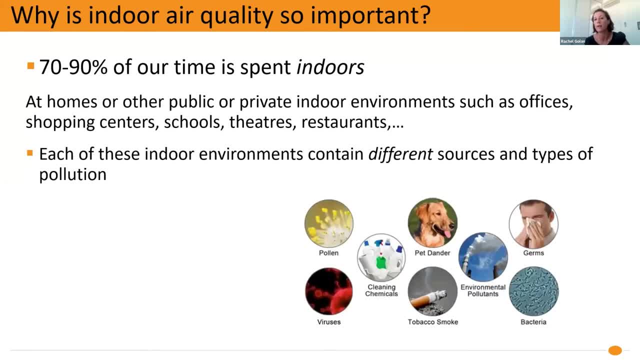 spending indoors, and it can be in our homes or in our other environments or offices, schools and so on. And again, as it has been said here, the indoor environments are maybe even more complex than the outdoor environment- I'm not sure- but definitely contain very 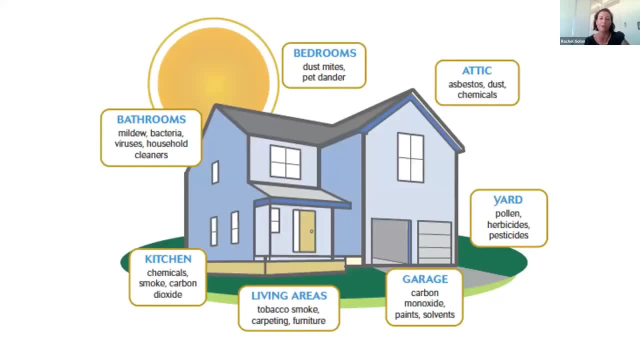 various different sources of pollution. Now I also put a little house here to show what we are exposed to in our houses, And it can vary, of course, from house to house. But, as we saw before in the talking, from the point of view of the outdoor environment And my 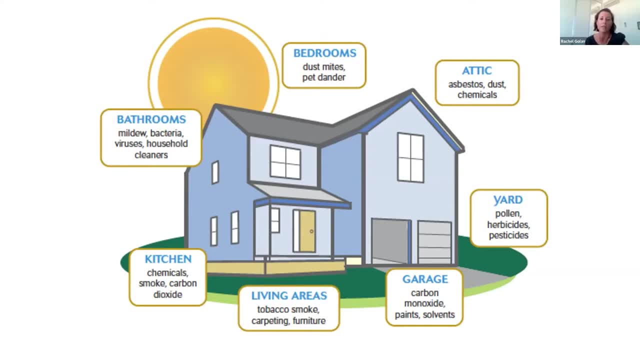 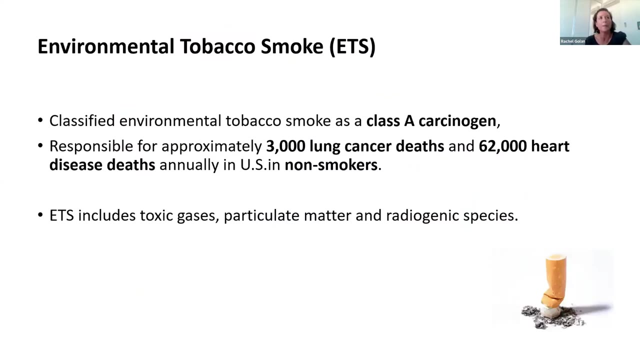 The home environment and office environment and other environments all include different types of pollution and substance that we are all to some extent exposed to, And this has also been mentioned before. but I must say that we can talk a lot about air pollution and air quality. 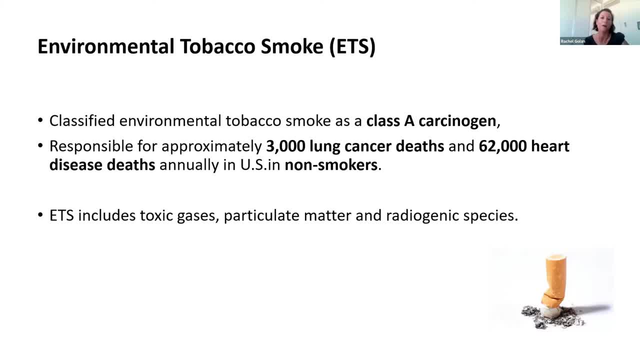 But, at the end of the day, environmental tobacco smoke, which is the smoke that we inhale non-smokers between us, is one of the maybe largest pollutants that we are all exposed to, whether we like it or not, whether we choose it or not. 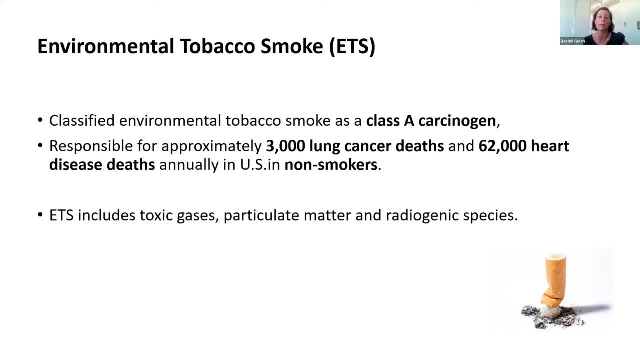 And also indoors, although many bans have been done in many places indoors, still we find, even in school children here in Israel, that all that, Although they do not come from a non-smoking, from a smoking household, they also show cotton in their blood. 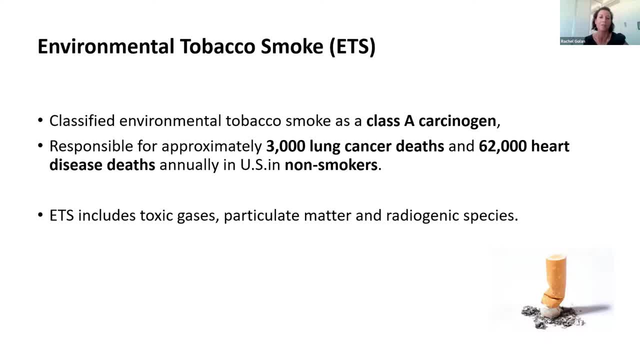 So we can talk a lot about very different kinds of sources, but at the end of the day, one cigarette can really expose us to a lot of indoor pollution, And we need to also always, I believe, mention this as well. And then this happened. 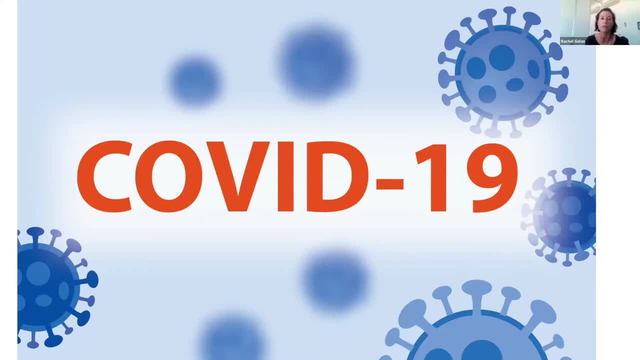 And the 70 to 90% time that we spend indoors changed to nearly 100% for many lags of times here in Israel, in other places around the world, And the indoor air quality, of course, has become more, much more of a problem to all of us. 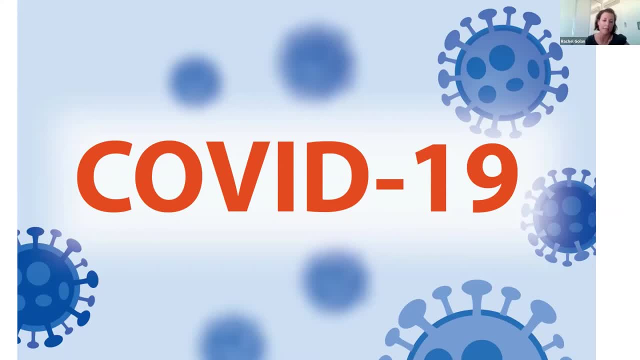 And we can see it also now in papers and studies that have been conducted and devices that have been talked about. suddenly, indoor air quality has become maybe more relevant, because everyone is talking about it. Everyone is talking about staying at home and what this brings to us. 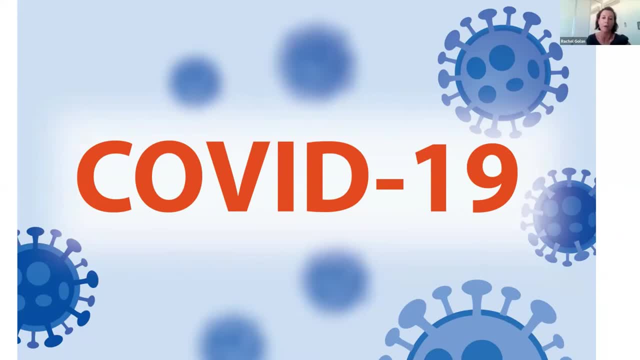 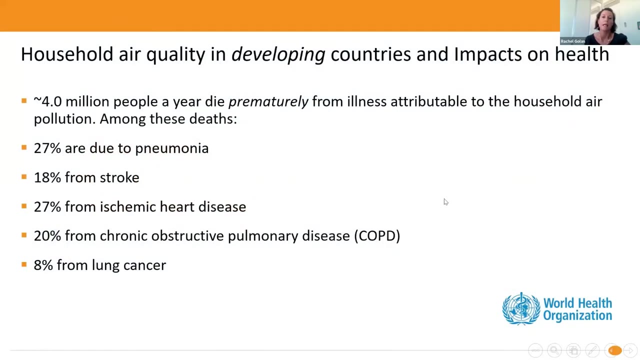 And there's so many effects of staying at home besides air pollution and air quality, But this is just another cherry on the top when we talk about staying at home, So this really brought the indoor air quality even more up to the surface. Now we've been talking a lot about indoor air and our houses, and we both brought here big houses. 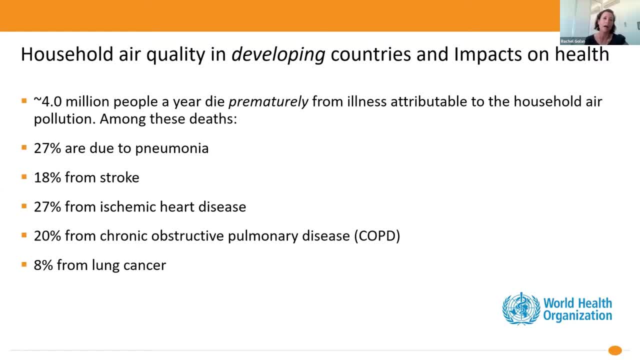 and nice houses. but we cannot talk about, I believe, about household air quality without looking at certain parts of the world and when we talk about the health effects of air quality and any of us who will do a literature review or try to see what comes out when we look about, 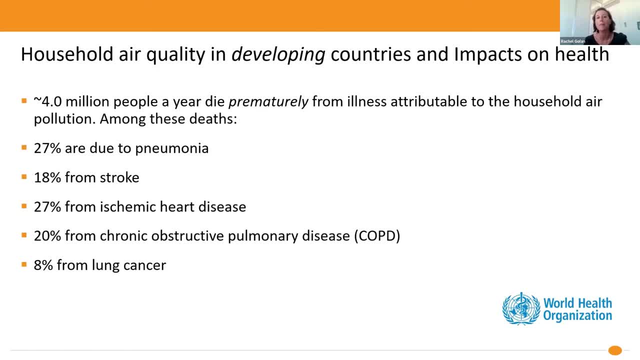 air quality, household air quality and health. many of the papers that will come against us first will be those coming from developing countries, and the numbers are always just too hard to really embrace. but I really believe that we cannot look aside when we're talking about indoor air quality and numbers that are coming from the WHO. 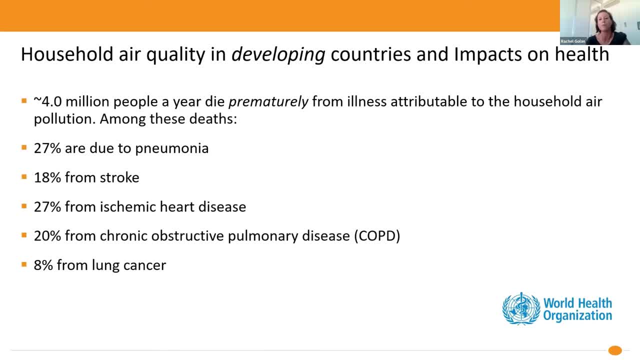 talking about over four million people per year who die prematurely from illness attributable to household air pollution, and this, of course, has effects on different societies and different populations, and when we're talking about developing countries, we are talking about mostly about open fires in huts and in small houses. 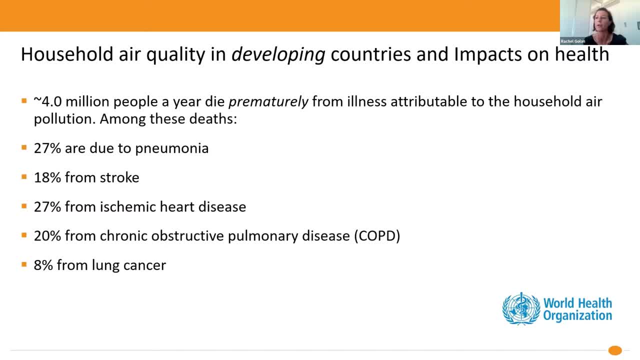 and any of us who traveled around the world a bit- in Africa or in Asia, we've seen these things and it's part of household air quality and the numbers of the effects on health, on our health and on these different populations health. you can see here in the numbers 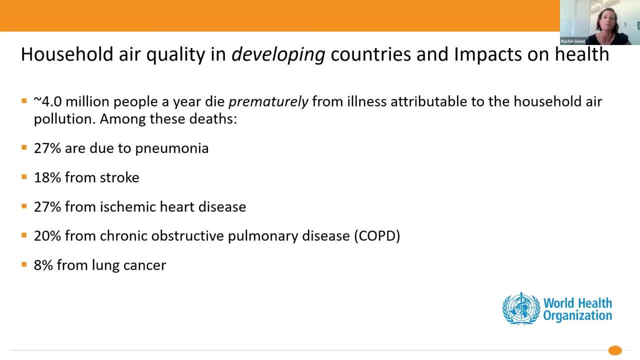 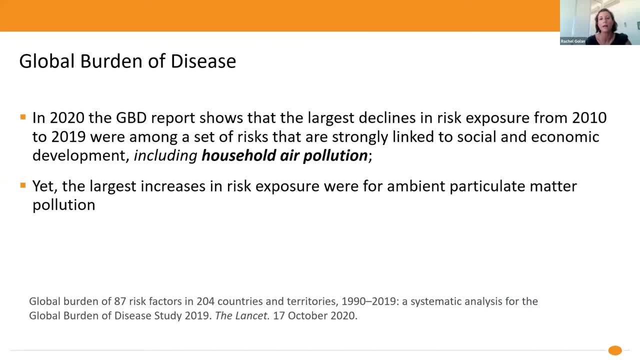 and most of them are cardiovascular disease and respiratory disease. the global burden of disease. the last report that made us actually do a systemic review about- and it was published last year- looked at the decline in risk exposures between the last decade, from 2010 to 2019, and they actually mentioned there that, among the set of risks that has 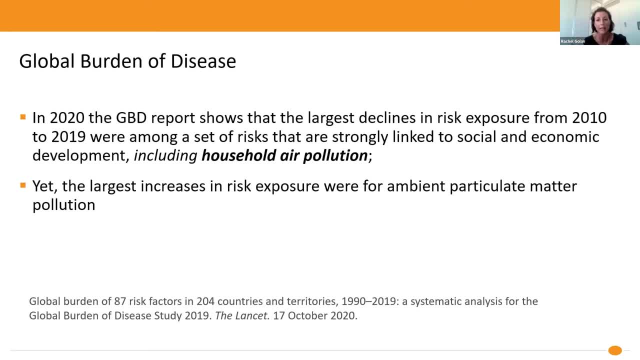 strongly that has actually reached the caribbean air quality chart, reduced and declined during this decade- is also household air pollution. but yet in the same report they also mentioned that the largest increases in risk exposure were for ambient particular matter. So I mentioned the open fires and the household air quality in places. 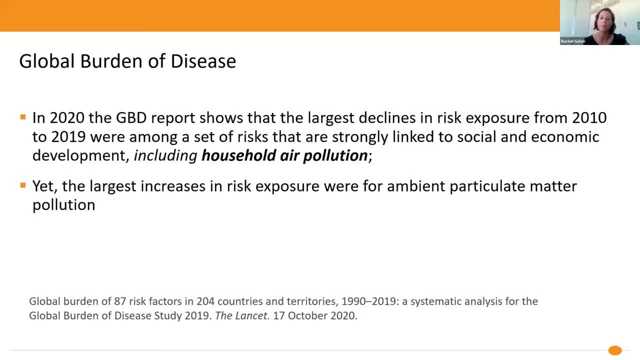 that we call developing countries, but we also talked here before about the increase, about the filtration into houses and how the outdoor environment influenced the indoor environment, and from this report we see that the fact that ambient, particular matter pollution is in rise. this, of course, is connected to what we are feeling inside our homes as well. 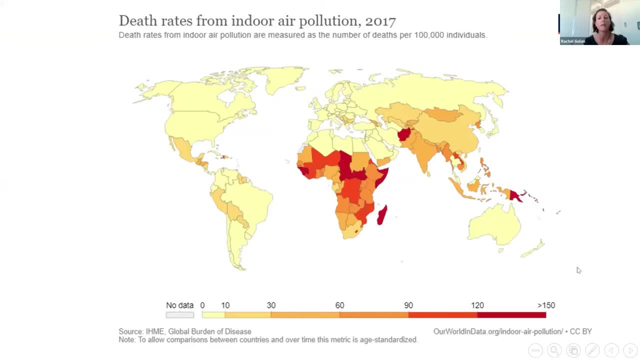 And again, still talking about the developing countries, I think this picture really shows us this global burden of disease and death- you know, Because what you can see here is from 2017- and death rates from indoor air pollution. And it is true that most of the red spots and the orange spots and the burgundy spots 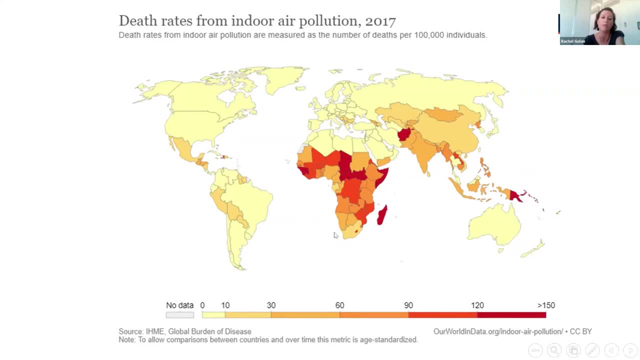 are around the areas of the African continent and Asia and a bit of Central and South America, And probably when we think about the way houses are built there and life is being held in those places, you can understand that probably most of this air pollution is coming from the different ways that open fires and fuels and so on. 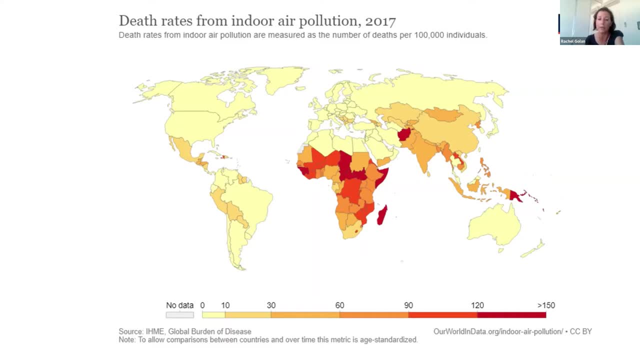 that we did not really talk about today And I'm not going to elaborate upon this, but this is still something we need to keep in mind when we're talking about health effects of indoor air pollution and attributable deaths- and you can see it here- But if we're talking about 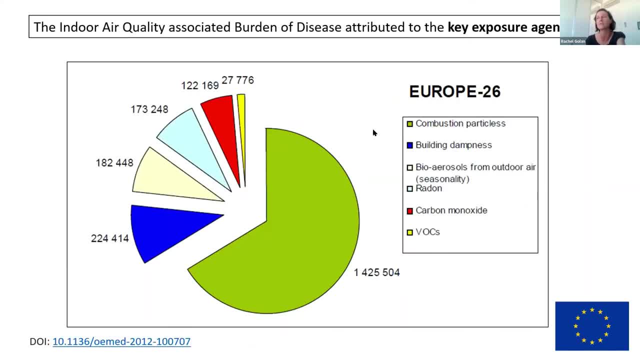 moving to what is maybe called developed countries, and we can look here at data coming from the European Union, and I will show you now three charts that look very similar to each other, but the legend is different. But they all are linked, of course, to each other. 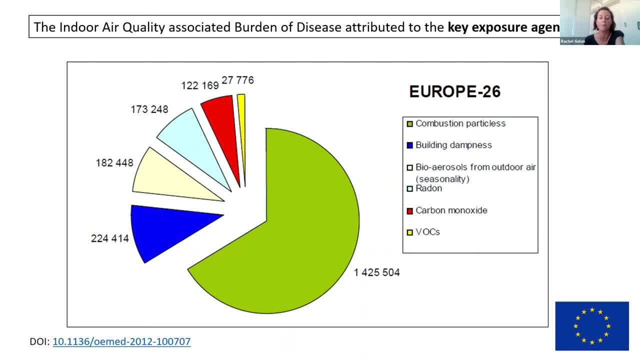 And here we can see the key exposure agents that are actually influencing indoor air quality and the different countries in Europe. And we can see here that the large effect, of course, is from combustion particles, but there's also other exposure agents that come from other sources. 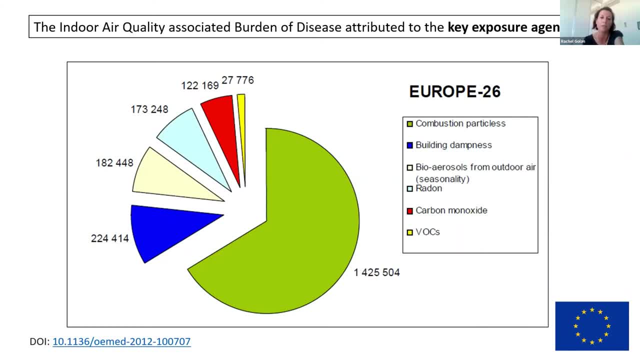 and some of them of course were mentioned here before and I won't mention them again- But when we try to see what are the sources of these exposures, so again, the green part here of the pie really corresponds nicely to the purple one here. 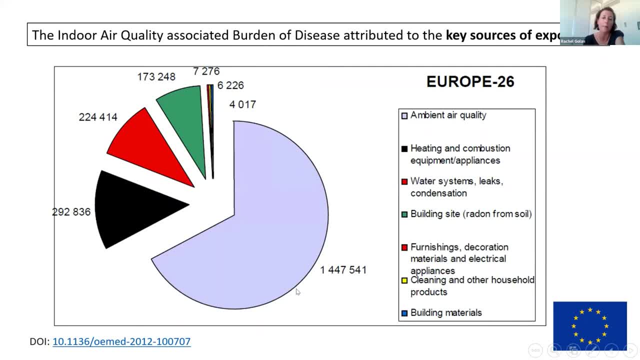 And the main source here is ambient air quality, But of course, as we said before and was mentioned also, there's other sources of exposure. that is more part of what's happening inside our houses, if it's, for example, heating or our water system, furnishing and etc. And if we turn from here to 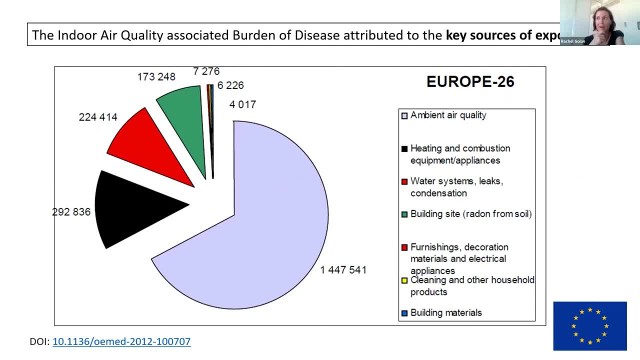 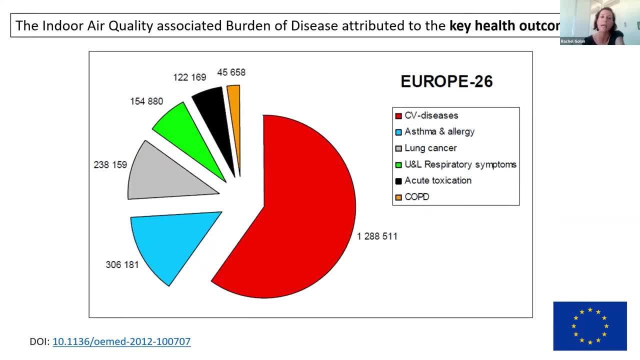 how it affects our health and, as mentioned again before, why do we actually care? We care because there is an association between the air quality in our homes and our health, And this is why I guess most of us care about what's happening in our indoors, Because, again, you can see the red. 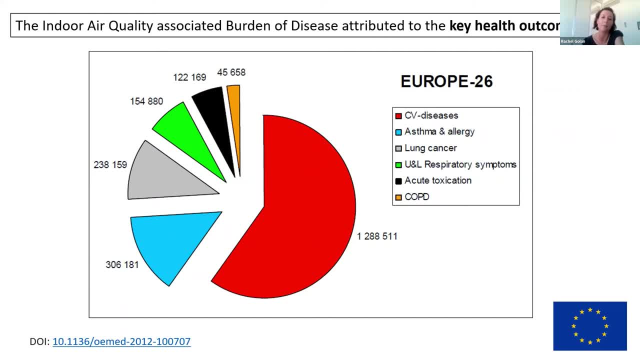 part of the chart here that corresponds very nicely to the green and purple that we saw before, And this is actually the health outcomes of cardiovascular disease. that today is really, as we know, is a very important part of the health outcomes of cardiovascular disease. 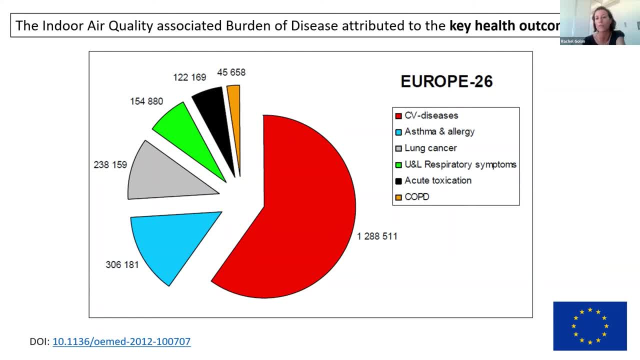 The second leading cause of death in Israel and the first leading cause in many countries around the world, And really the connection here to both the ambient air pollution, but definitely also to indoor air pollution, is very clear from this chart And we can see this across. 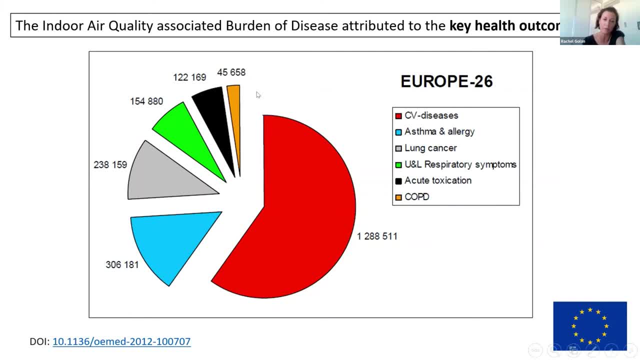 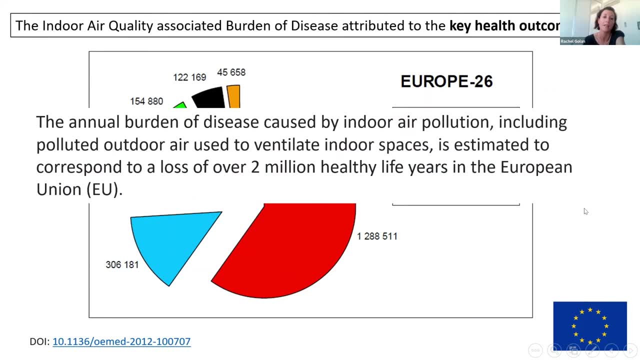 Europe, And, of course, other respiratory diseases, of course, are also connected and associated with indoor air quality. The annual burden of disease caused by indoor air pollution, including polluted outdoor air used to ventilate indoor spaces, is estimated to correspond to a loss of over 2 million healthy live years in the European Union. 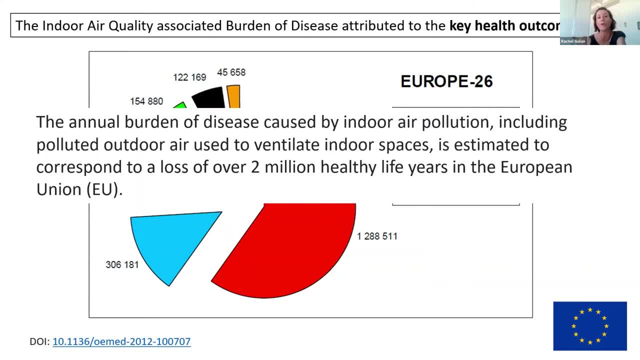 annually. So if I showed before the map of the world and most of the red and orange spots were coming from places other than Europe, these numbers are also quite disturbing for us when we think about the effects of health, of air quality in our homes and in our environments, and how it affects our health. 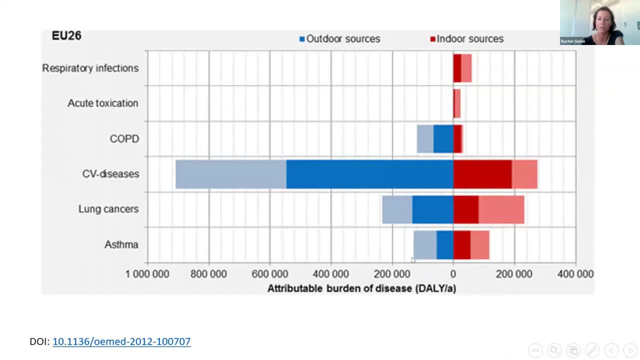 I like this chart very much because I think it really shows the combination of both sources, the outdoor sources and the indoor sources, And, as I mentioned before, we know a lot. there's a large body of evidence that shows the connection, the association between outdoor sources, ambient air pollution. 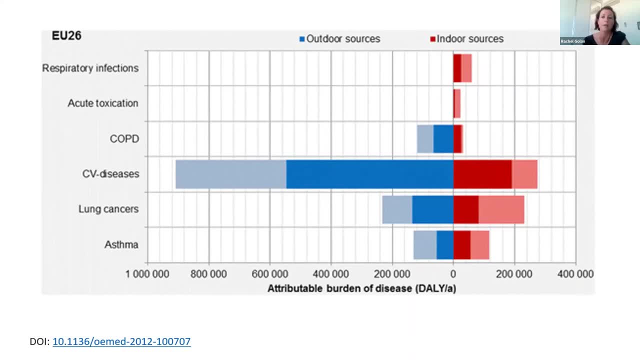 and cardiovascular disease and other diseases, respiratory disease, like we can see here in the blue charts here on the left side of the slide. We cannot blind ourselves to what's happening here and we can really see that indoor sources are a large contribution to cardiovascular disease and to other diseases. So it's very 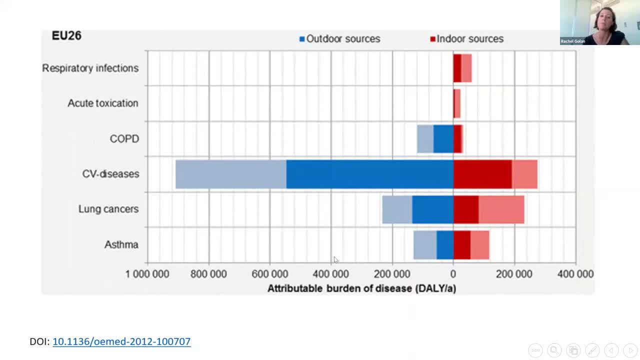 easy, I think, to look at what's happening outside. We know it's much easier- I won't say it's easy, but it's much easier and much more developed- the way that we measure what's happening outside And if we talk about regulation. 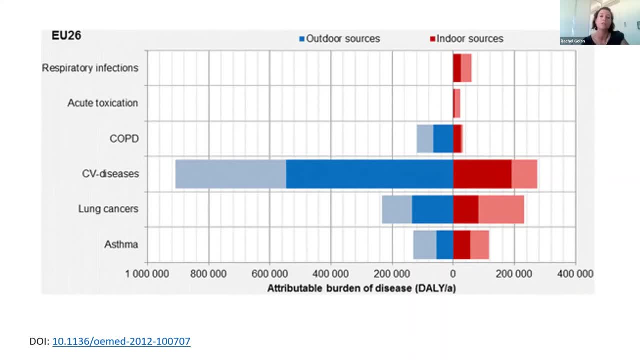 it's maybe even easier or doable to have regulations about what's happening outside, And I think what I mentioned now is what makes indoor air quality, the health effects of indoor air quality, much more cumbersome, because it's difficult to measure it. it's difficult to measure the effect on our health, but still we cannot ignore it. 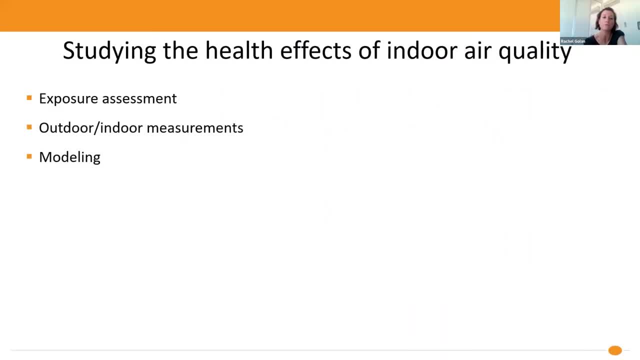 and we've seen it in the charts that I've just shown, When we're talking about studying the health effects of indoor air quality, and we've seen in the previous talks a lot about exposure assessment and the filtration between the outdoor and the indoor and how they correspond these measurements. 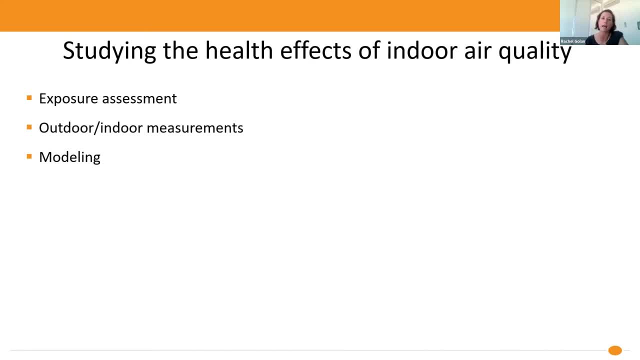 and of course there's the modeling. but when we try to put inside and each of these, of course, methods are not simple And then if we want to combine the epidemiology inside everything and really look at the health effects, this is also a difficult question to answer. 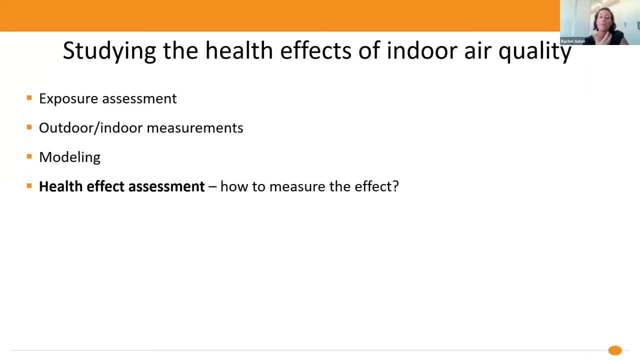 How do we measure the effects? How do we measure what's happening in our bodies? Does anything happen in our body at all? Going back to what Professor Bridgman said in her EHB paper that was mentioned, it's very difficult to measure the effects of indoor air quality. 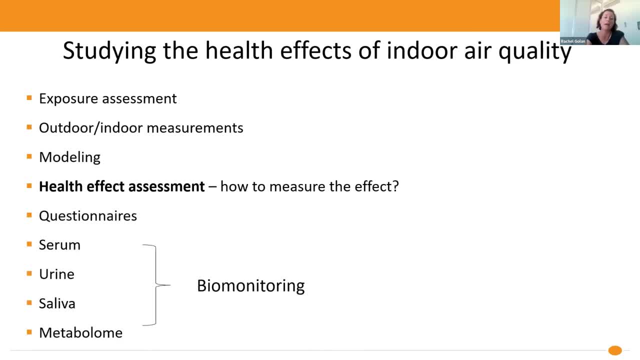 That was mentioned before. Why do we even care? Does it really affect us? And, of course, there are questionnaires and we know the questionnaires are good and easy, maybe to implement, but are very prone to bias and the data that we can get. 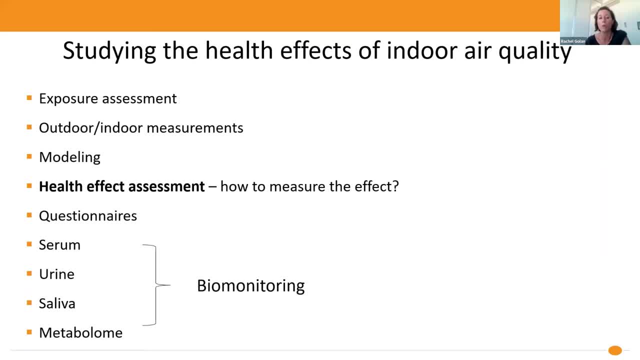 from questionnaires is sometimes not so informative. But of course we have today, and as mentioned also before, all the issues of biomonitoring in the last decade, even in the last few years, even if you're talking about here in Israel. 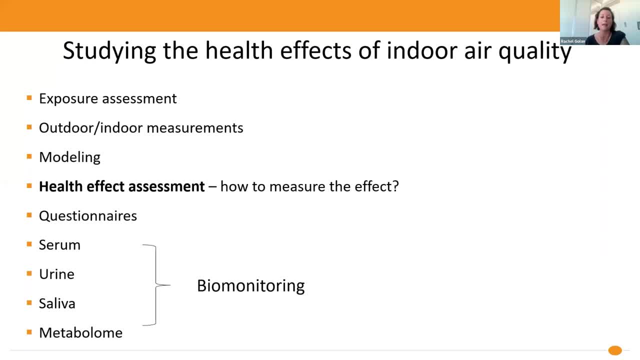 about my biomonitoring. that has been really expanded and advanced and biomonitoring is done also in studies here in labs here in Israel, but still this imposes a big problem for studying, since, of course, when we're thinking about people, children, 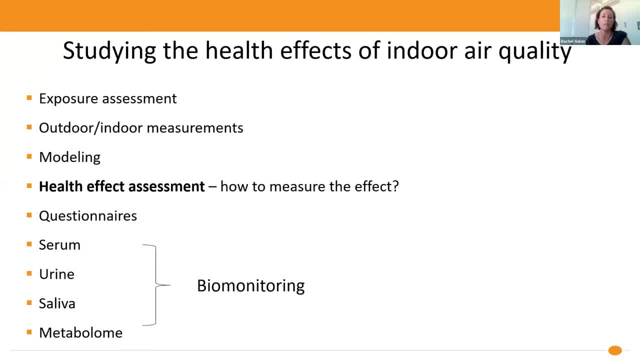 adults. biomonitoring is not something that's so easy- Ethical issues and also people who would be happy to participate in these kinds of studies. but still the biomonitoring is getting more and more advanced and with the metabolomics it's also being more and more advanced. in the last five or ten years, I think, the health effect 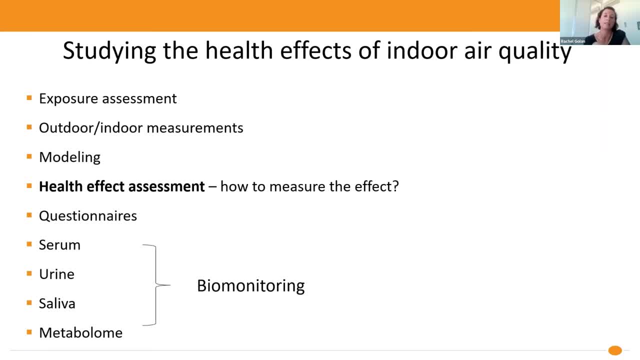 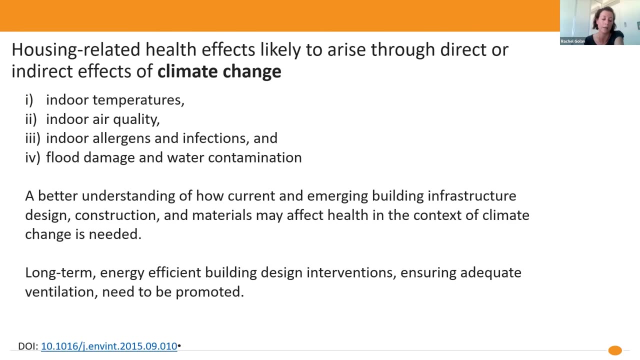 assessment is getting much more better, but still it's, of course, very expensive and can be very and difficult to implement in different kinds of populations, But this is, of course, something that we need to consider when we're doing a health effect assessment. 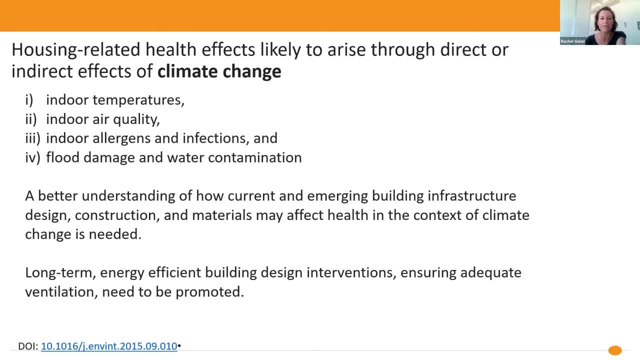 One minute left. Okay, I would like to with the one minute I have just to raise two things that I would like to talk about when we're looking forward- And I cannot finish the talk without talking also about climate change, because I don't have to say anything to this audience about climate change- 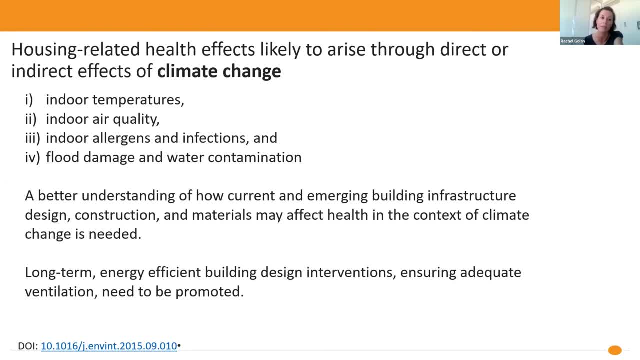 but when we think about it in terms of how it will affect our indoor environments if the temperatures will raise our air quality, in indoor allergens and infections and flood damage and water contamination. all these things we need to keep in our mind and we can use it as a discussion. 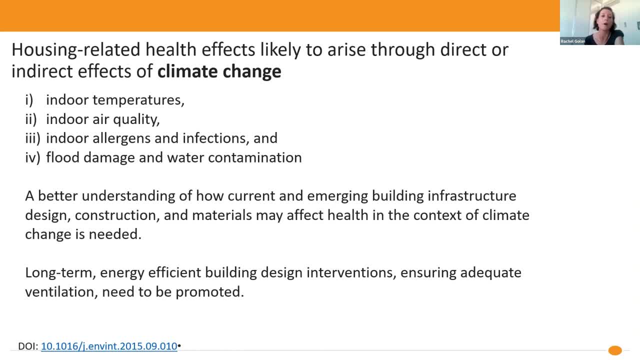 point And we really need to understand how current and emerging building infrastructure design, construction and materials may affect health in the context of climate change, and we really- and this was mentioned also before in the talks- when we think about how buildings are designed today, what materials are used today- many times it's talked from: 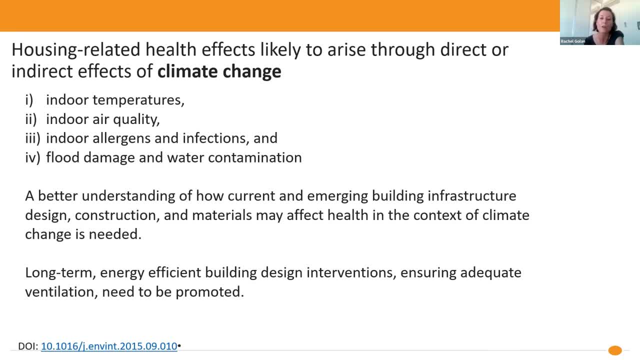 the perspective of engineering, but we also need to keep in mind the person who lives, the people who live inside the house, and how the way that houses and buildings are built will also take into consideration the effect of air quality and the health of people. 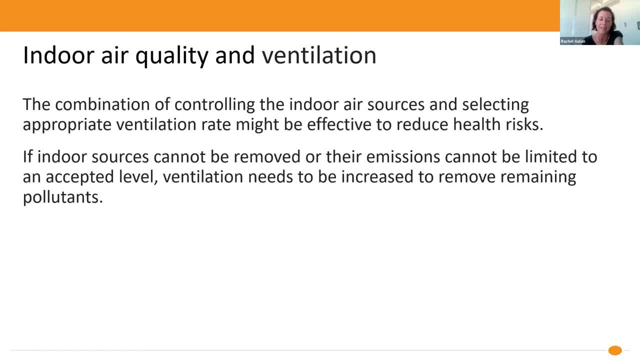 And this was mentioned and I was really happy that it came up- and this is not my area of expertise, but I do believe that in some points, in some things that we are exposed to, for example- and I'll take something which maybe is much easier to embrace- when we're talking about nutrition- 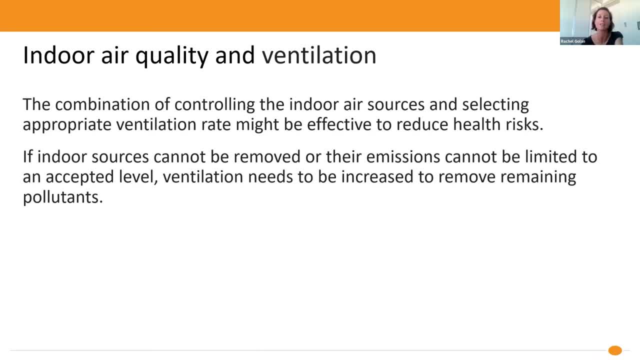 for example, we can do many things in terms of teaching, putting regulations and teaching the populations of how to reduce different substances, how to reduce different substances, how to reduce that we do not want them to enter our bodies. But in terms of indoor air quality, sometimes we 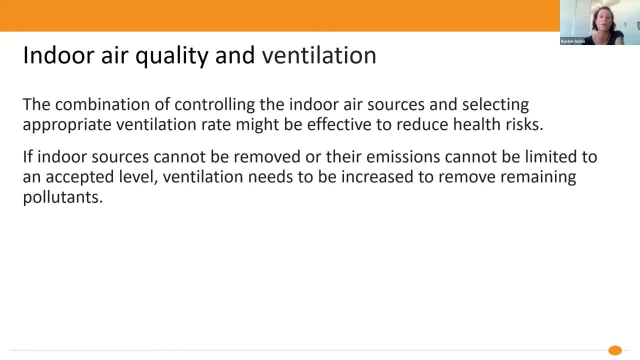 do not have, we probably won't have the best solution for how to really stop the pollution and stop the indoor air quality from being not so optimistic, and therefore ventilation is something that I really think that we should think about specifically when we talk about the health risks. 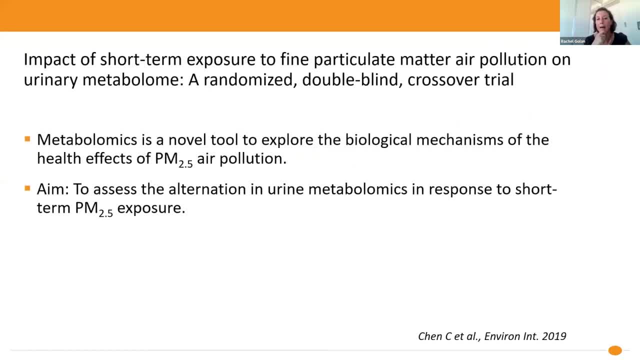 and I don't have time for this, but this one little paper that I brought here that talks about this exactly, and it was published two years ago. it was in China, in Shanghai, among students, where in a randomized double-blind crossover trial, they used real or sham indoor air. 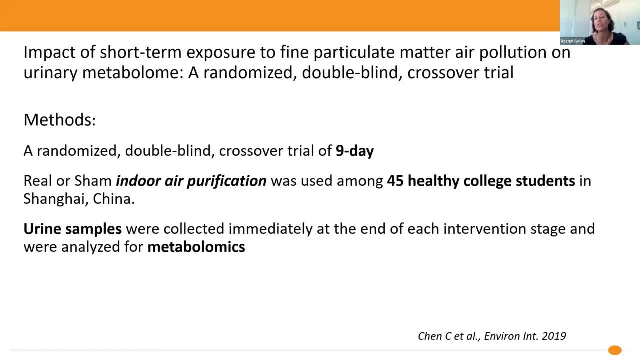 purifications for nine days and they collected urine from these students, from these college students, and they collected urine from these students, from these college students, and they and they compared the urine between the days where there were purified air and non-purified air. 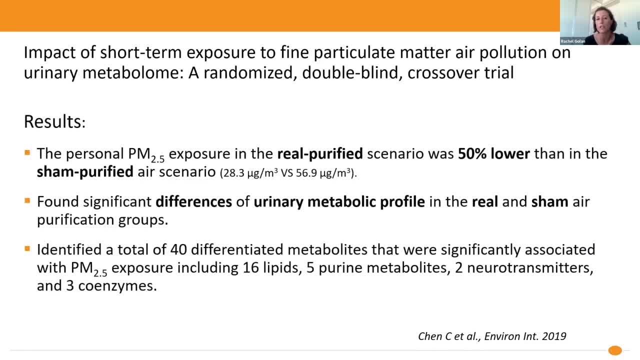 and they saw very nicely that the exposure, of course, was decreased and they could see it in the urine and the metabolic profile. they used the metabolomics that I mentioned before. they used it here and they really found a difference between students who were exposed to. 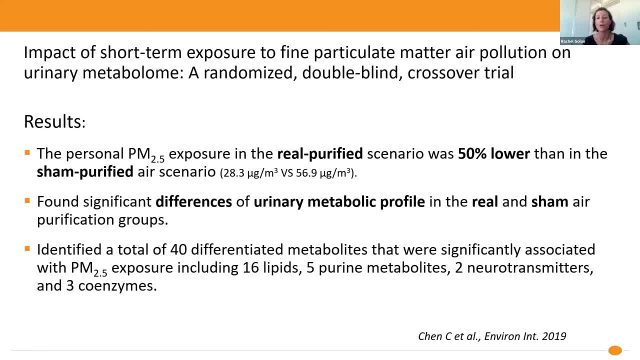 air that was purified and air that was not purified. So well, this was my. I'll finish. my time is up and I'll be happy to take questions when we have time.